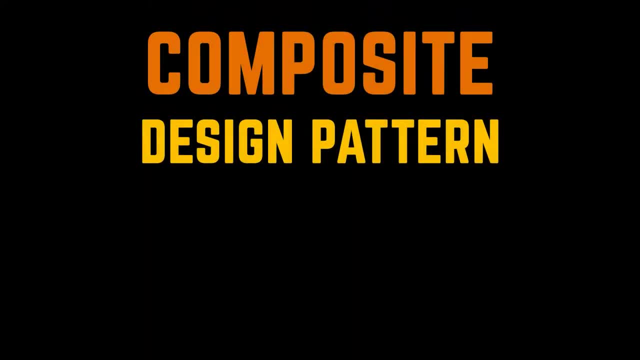 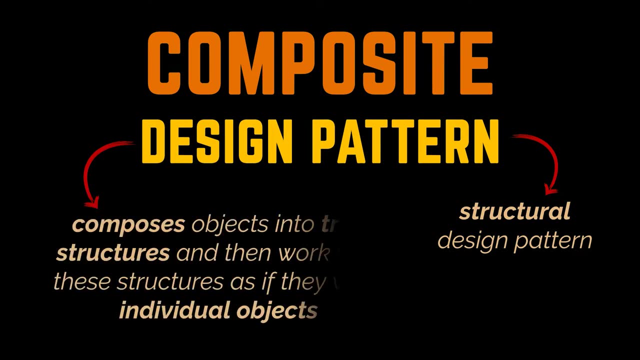 The solution to these problems resides in applying the composite design pattern. The composite pattern is a structural design pattern that lets you compose objects into tree structures and then work with these structures as if they were individual objects. You see, using the composite pattern makes sense only when the model and object structures 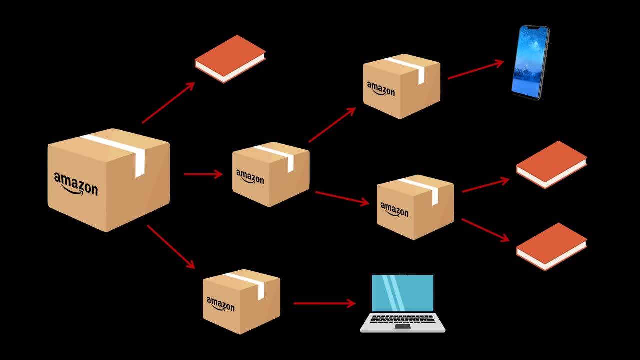 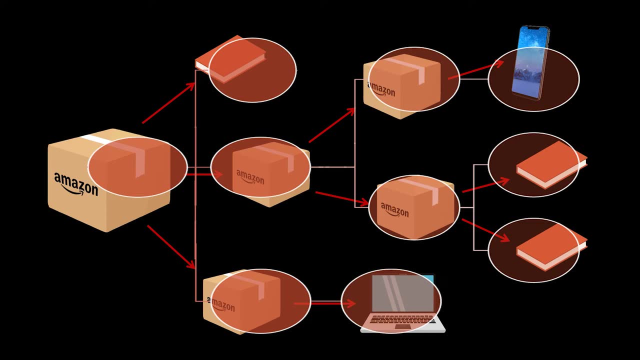 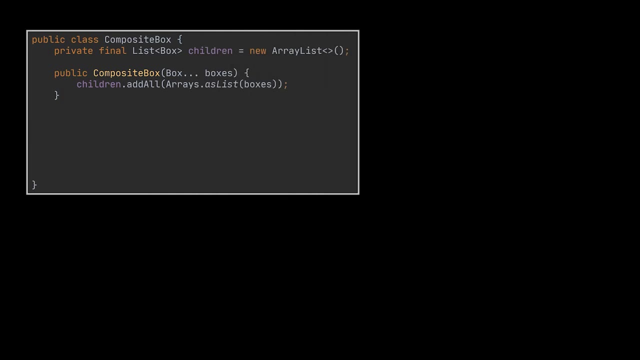 of our application can be represented as a tree, And if you take a look at our previous representation of this example, you will see that, well, it really is very similar to a tree structure. So to apply this pattern, what we are going to do is create a composite box class whose sole purpose is to store multiple 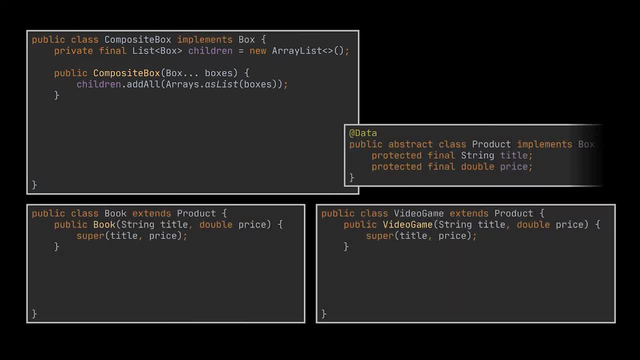 other boxes, Then let this class and the different product classes- which in this example will be the book and video game classes, let's say, implement the same interface. This interface, which is the box interface, will declare a method for calculating the 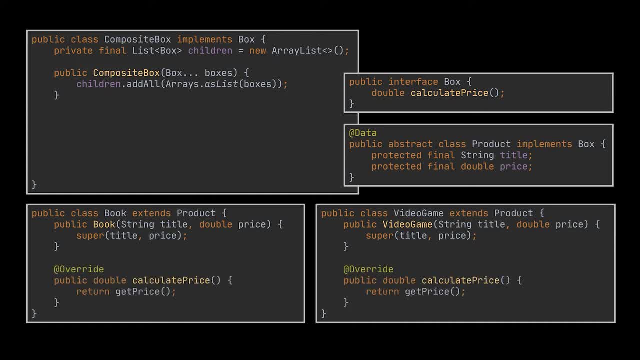 total price. Now, in our product classes, this method's implementation will simply return the product's price. But for a composite box it will iterate over each item in the box, ask its price and then return a total sum for this box. 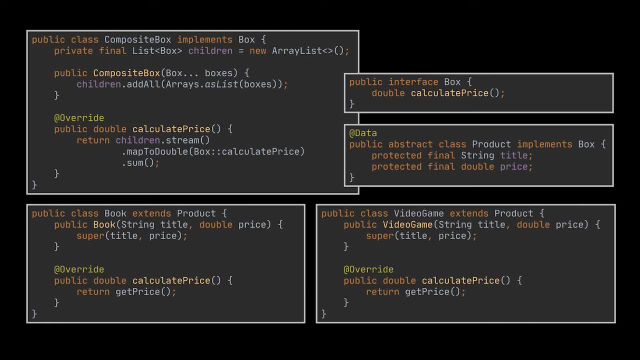 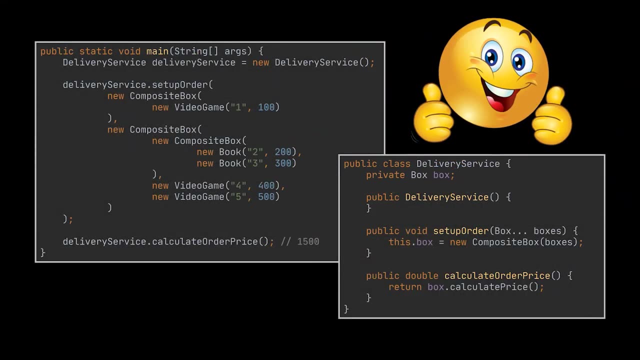 If one of these items is a smaller box, that box would also start going over its contents until the prices of all of its inner components are calculated. A box could even add some extra cost to its individual price, such as a packaging cost. The greatest benefit of this approach is that you don't need to care about the concrete. 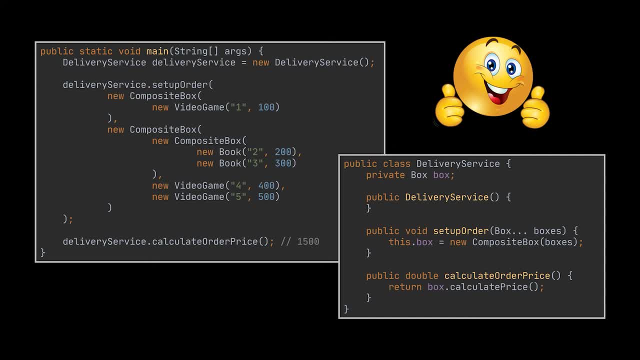 class of objects that compose the tree. You can treat them all the same way by making use of the common interface. When you call a method, the objects themselves pass the request down the tree. Ok, with this example in mind, let's take a look at the structure or class diagram of: 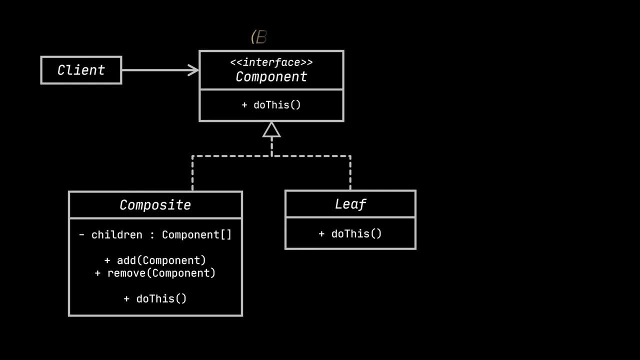 the composite design pattern. The first thing you may have noticed is the component interface, which was represented by the box interface in our example. This interface describes operations that are common to both. For example, if the component interface is a box, the object will be represented by a. 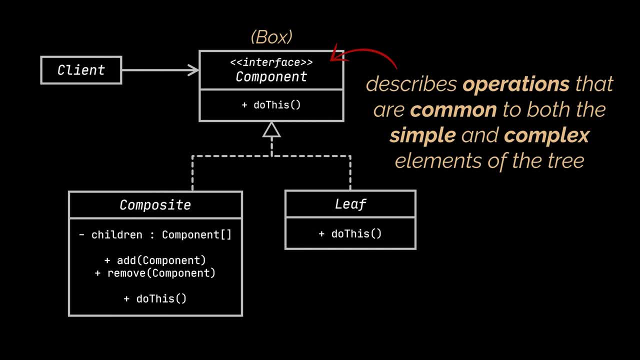 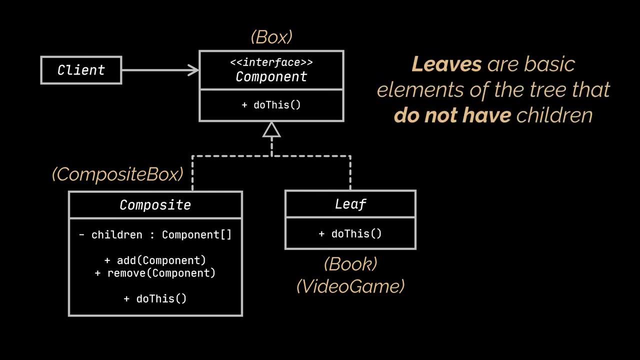 box. This means that the component interface represents the simple and complex elements of the tree. The next classes you can see are the leaf and composite classes, which were respectively represented by the composite box and different product classes we made use of. Leaves are basic elements of the tree that do not have sub-elements. 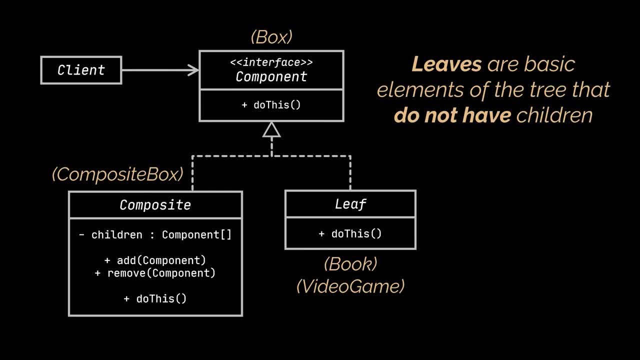 Usually, leaf components end up doing most of the real work, since they don't have anyone to delegate the work to. On the other hand, the composite, aka the container, is an element that has sub-elements, Leaves or other containers. A composite doesn't know the concrete classes of its children. 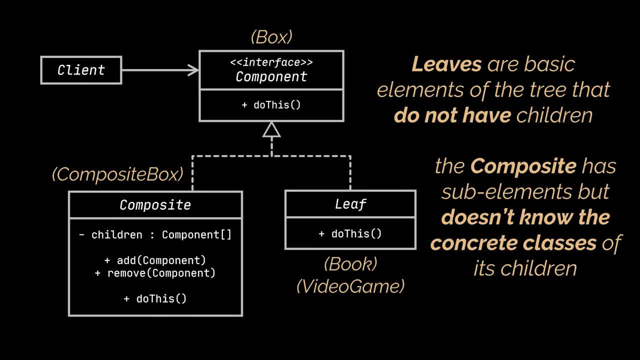 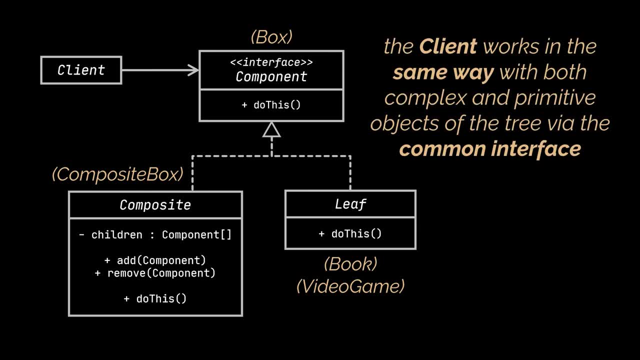 It works with all sub-elements only via the component interface. Now onto the last piece of this diagram, which is the client. The client works with all elements through the common interface we created, which means that he can work in the same way with both complex and primitive objects of the tree. 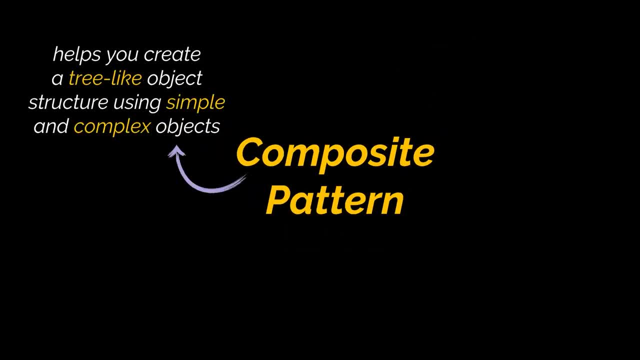 So, to sum everything up, The composite pattern helps you create a tree-like tree, A tree-like object structure, using simple and complex objects. To do that, both of these elements will have to implement the same interface, and by making use of this interface, the client will be able to treat individual objects and their compositions. 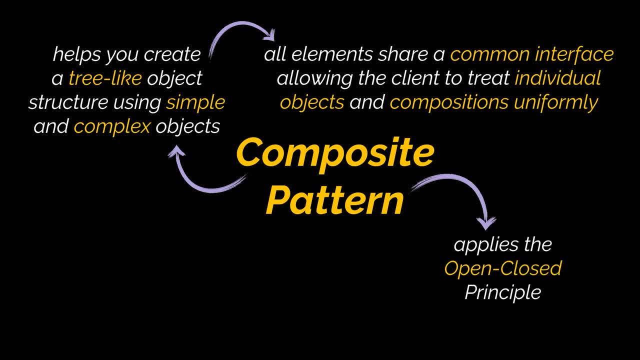 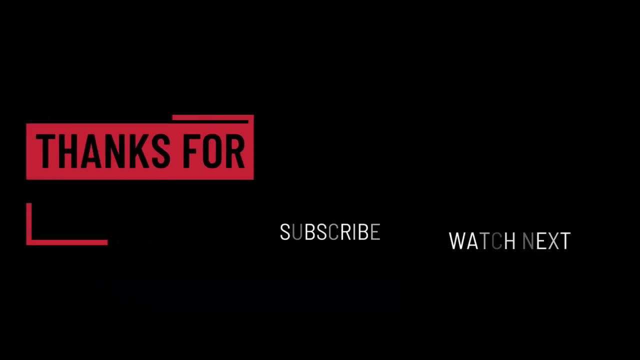 uniformly. Additionally, by making use of this pattern, you will be applying the open-close principle, because you can now introduce new element types or products, in our case- into the app without breaking the existing code. So That's it for this video. I hope it was helpful. thank you guys for watching. take care and I will see you in the next one. 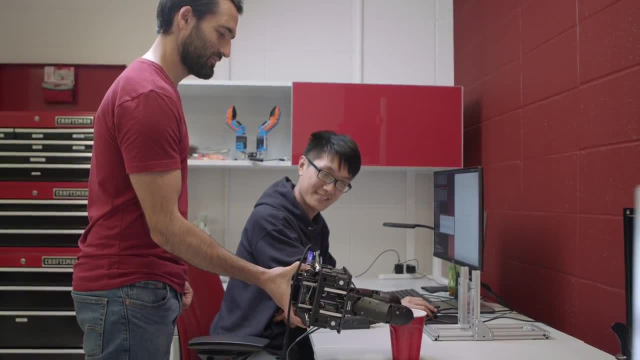 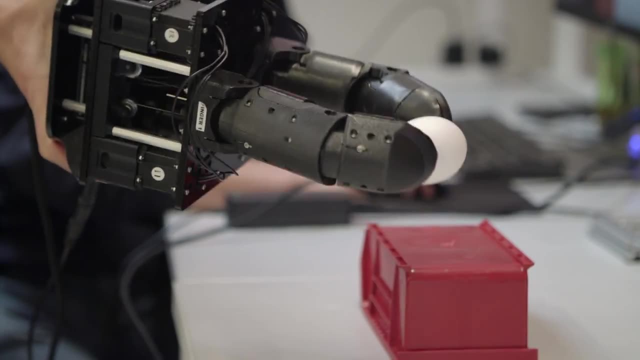 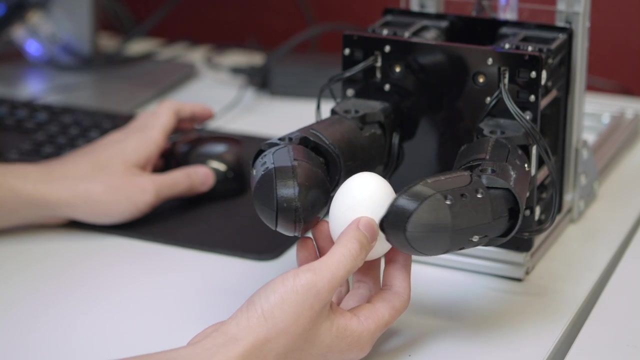 We're trying to get robots' hands to feel the way we feel. Your sense of touch relies a lot of information on where contacts are happening. If the object is slipping, you have that vibration on your fingertips that tells you that the object is about to slip and then you can take a corrective action. 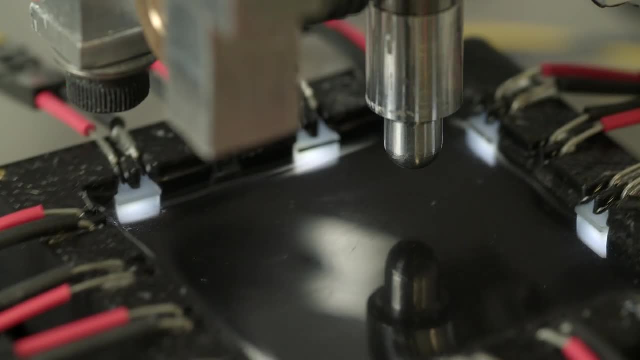 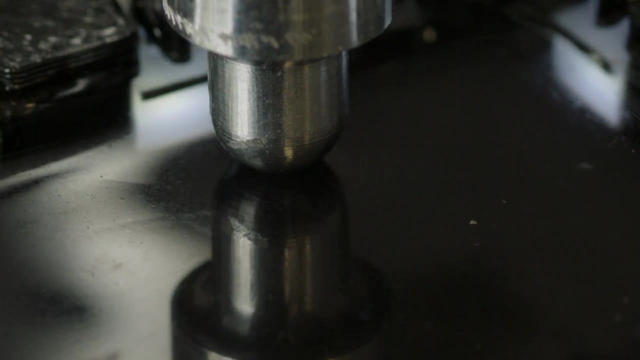 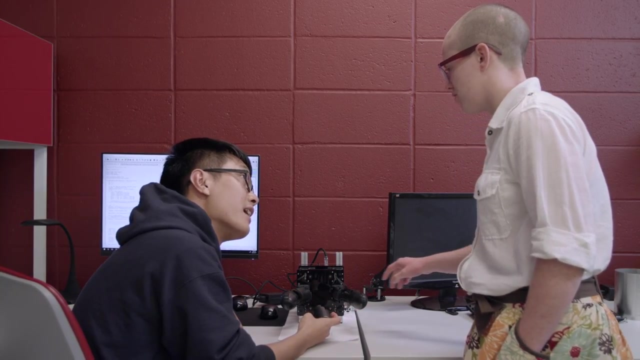 What we're looking at is one of the prototypes for our tactile sensors. So this machine just collects the data to build that model between the mapping of the signals we collect and our variables of interest. Eventually we want to have a rubber like this covering a robot hand. 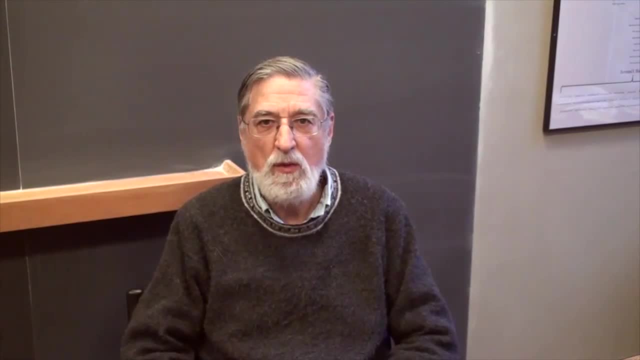 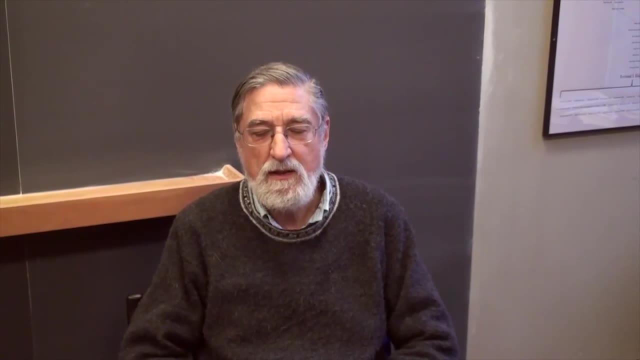 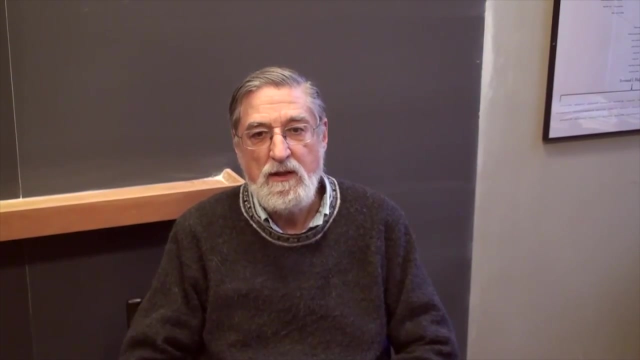 Well, I'd like to say a few more words about edge states and their role in understanding the quantized Hall effect. You've already seen how, for a system of non-interacting electrons, in the absence of impurities in a strong magnetic field, you can get a quantized Hall effect.